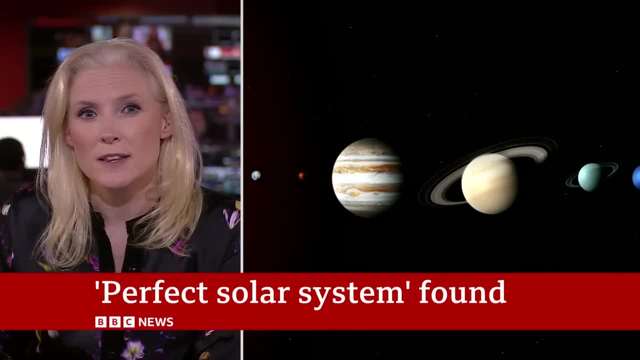 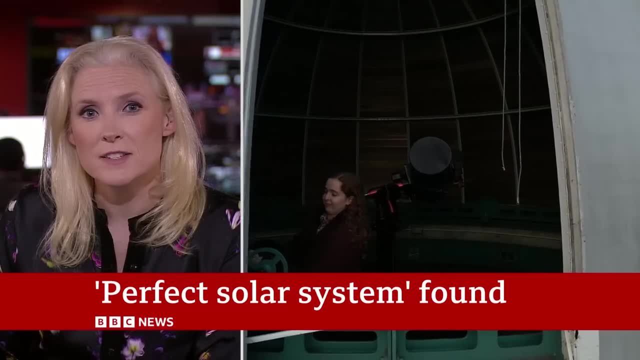 formation up to 12 billion years ago. These undisturbed conditions make it ideal for learning how the worlds were formed and whether they host life. Let's speak now to Pallav Ghosh. Hello, Pallav, Tell us what's up. We can hear from Pallav. 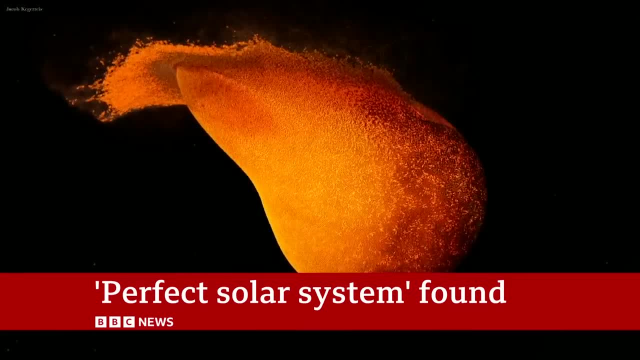 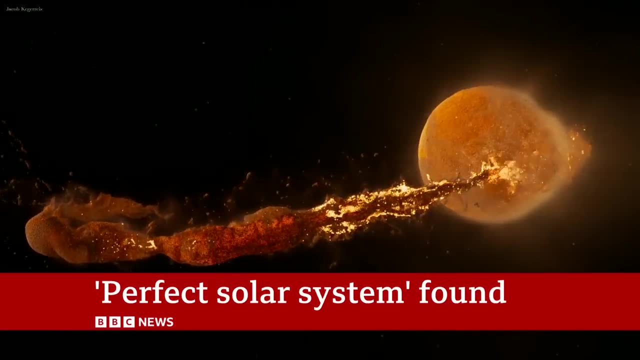 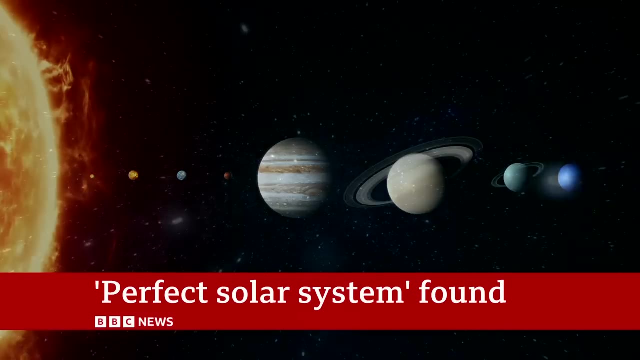 Ghosh. Here's his report. Our solar system had a violent beginning. Worlds crashed into each other as they formed, disturbing their orbits and eventually leading to the planets of vastly different sizes that we know today. But if we travel through space 100 light years, we find another solar system. 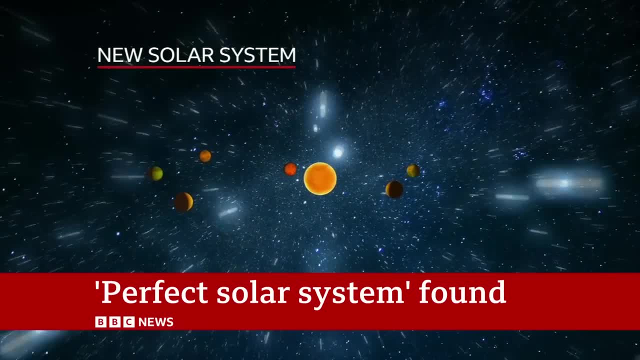 But what if we travel through space 100 light years and we find another solar system? but what if we travel through space 100 light years and we find another solar system and one that was created in much calmer conditions, without so many violent collisions? The system- 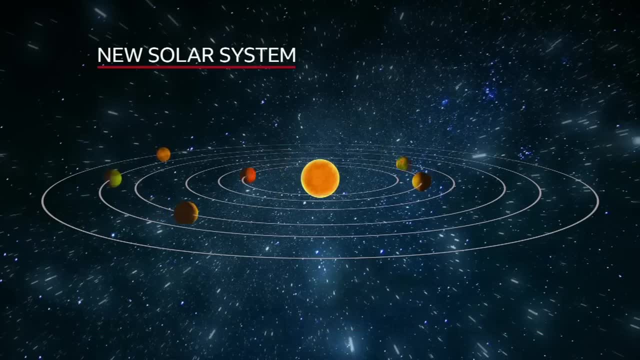 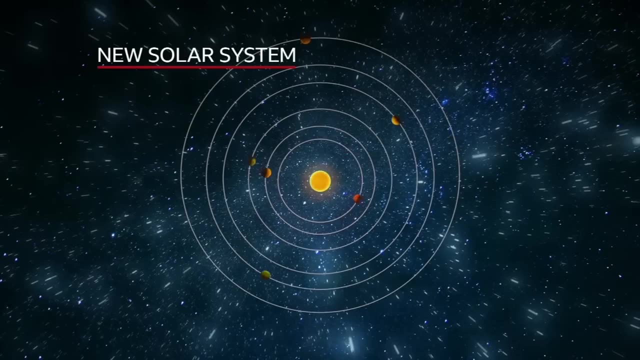 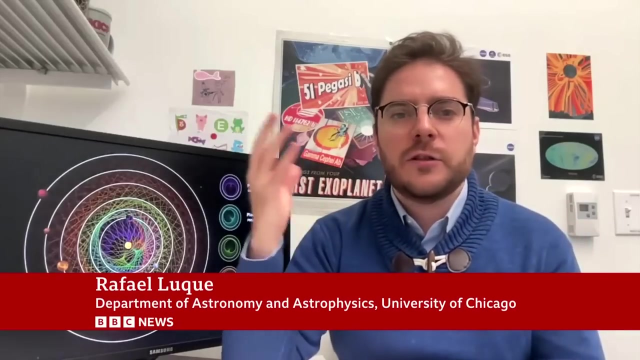 has six planets, all of a similar size. Their orbits haven't been disturbed and so are in perfect harmony. It also has a bright star that makes it easier to study their atmospheres for signs of life. This system has such unique properties. The star is so bright that it's 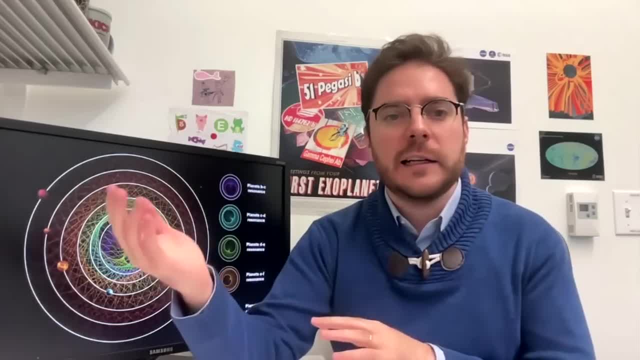 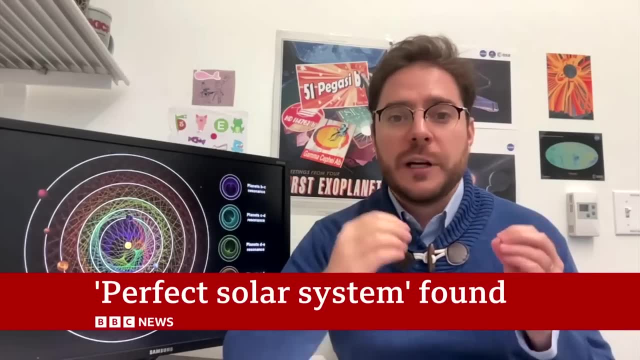 going to allow us to do so many studies from telescopes in the ground and in space, about their atmospheres, how they form, how they evolve, And we have never had the chance of observing such a bright system, with so many planets all at once, until now. 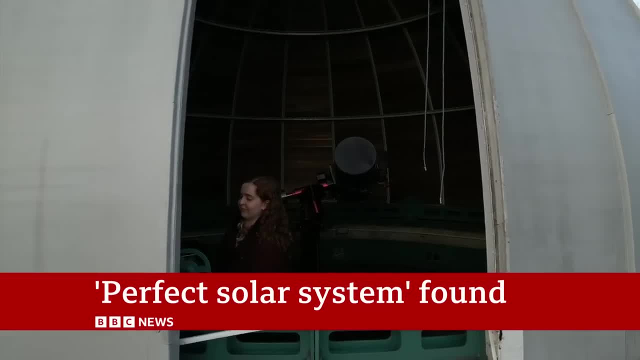 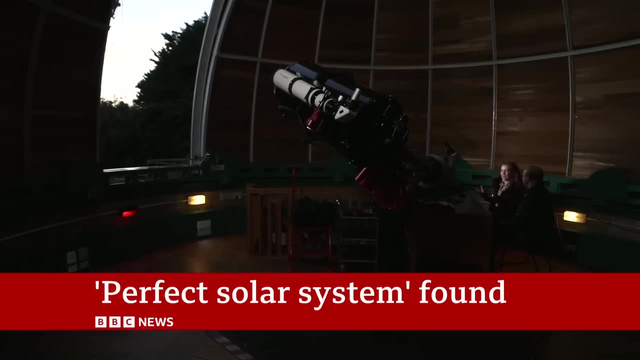 Astronomers have discovered thousands of solar systems in the past 30 years, but none of them are so well suited to study how planets formed as a newly discovered one. I think it just makes me really excited. Every day we're finding new. 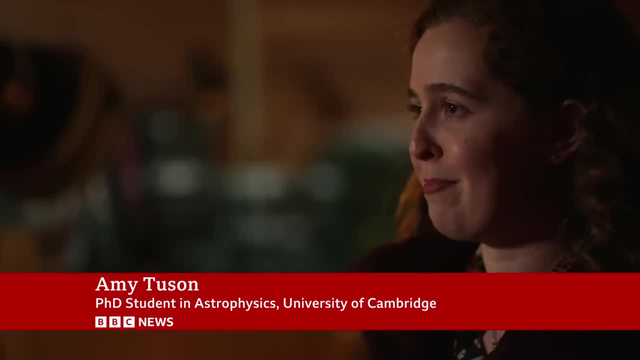 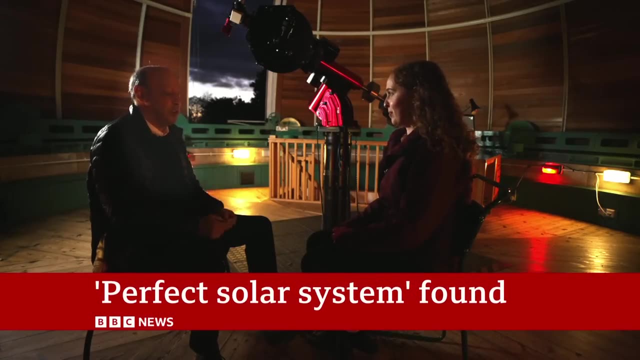 exciting things. We're finding systems that are going to allow us to learn more about these planets, that are going to test our models and our current understanding. So is this solar system the perfect solar system? because it gives you the perfect laboratory to find out how planets are created. 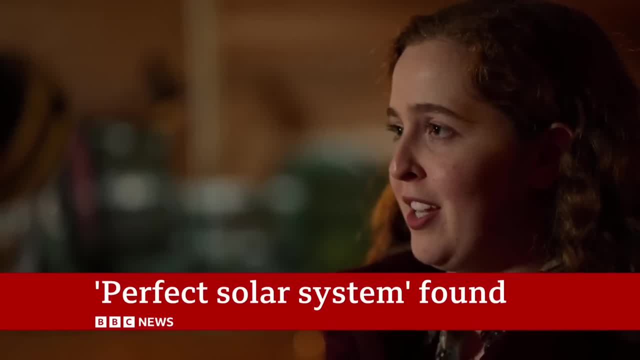 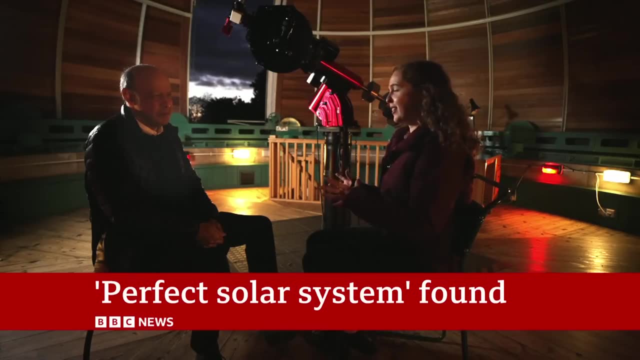 Exactly So. everything about this system is ideally suited for the information we need to find out. So we have the bright star. The planets are in a really interesting configuration, and because of that we know that nothing too dramatic can have happened over the billions of years since they formed. 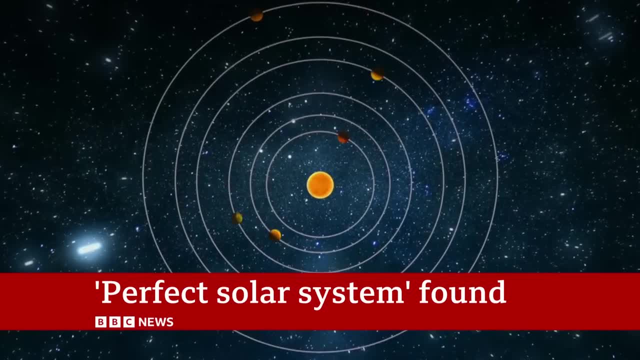 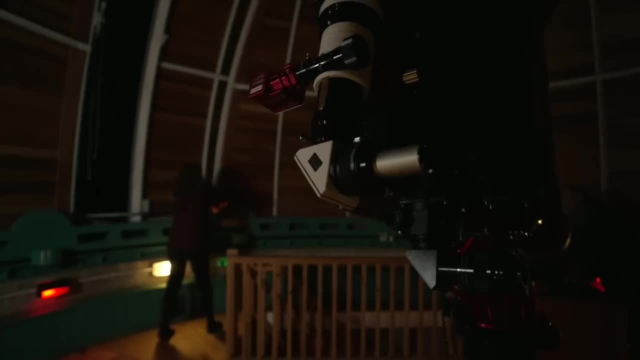 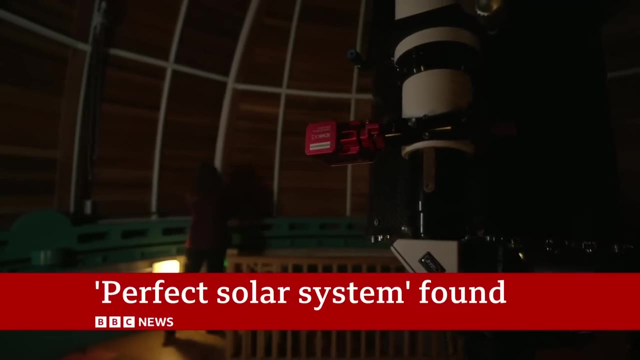 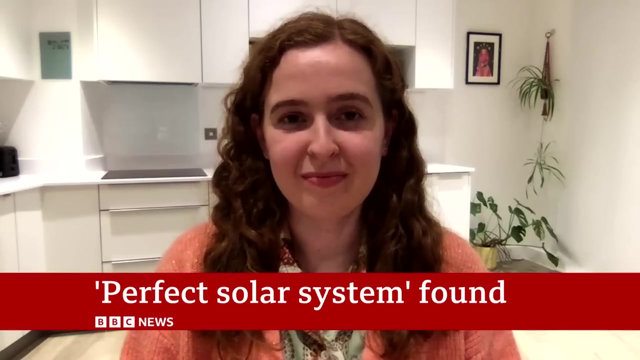 This perfect solar system, published in the journal Nature, will help astronomers discover exactly what these faraway planets are made from, how they evolved and, critically, whether they may be home to life. Pallab Ghosh, BBC News, Cambridge. Well, let's speak now to Amy Toussaint, who you saw in that report, a PhD student who's the author of the paper about a new 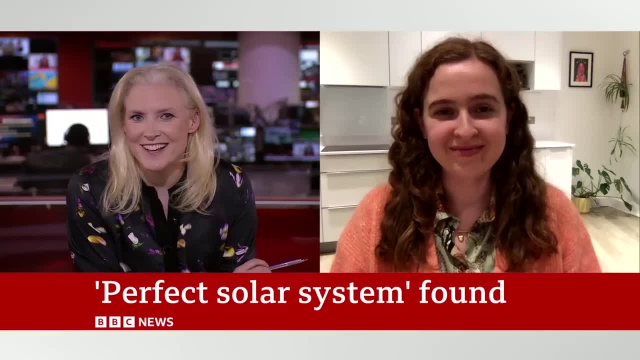 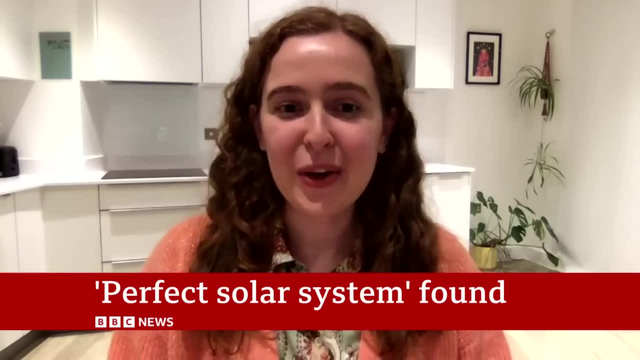 solar system. She joins us now from Cambridge. It's lovely to see your enthusiasm there, Amy, in that report. It's clearly very exciting times, isn't it? Just explain to us how you discovered this. Yes, So this system was a really big international effort, working with telescopes from NASA and ESA. 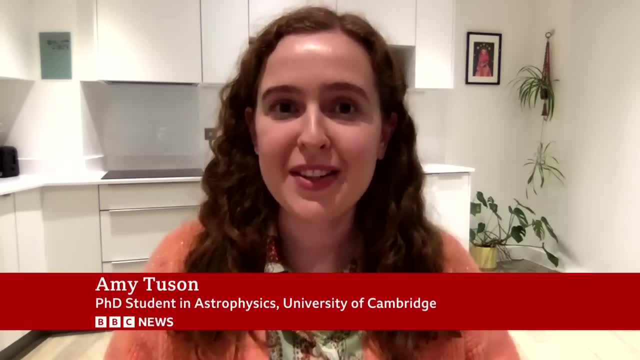 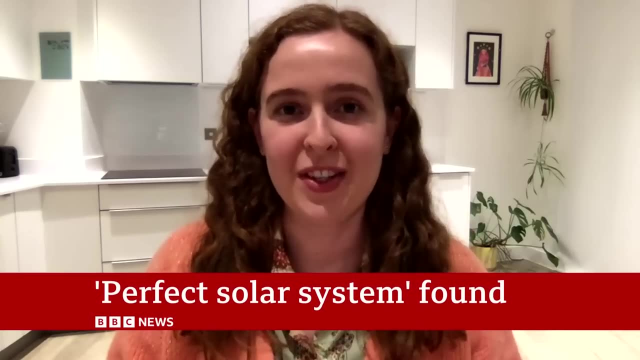 So we discovered this system using what we call the transit method. So we're looking at these stars for the telltale signs of exoplanets which cause small drops in the star's brightness. Yeah, So this is just yeah. what does that mean? 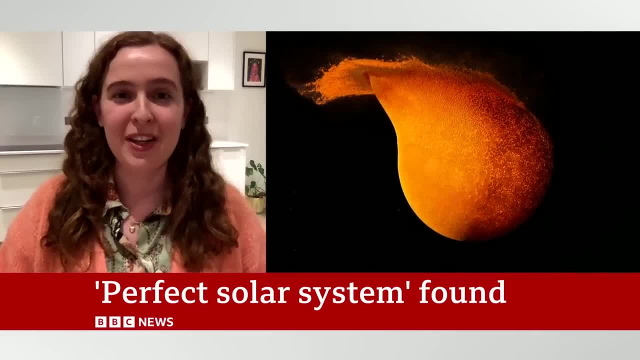 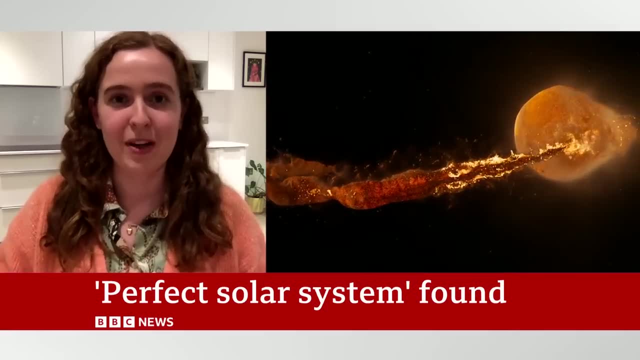 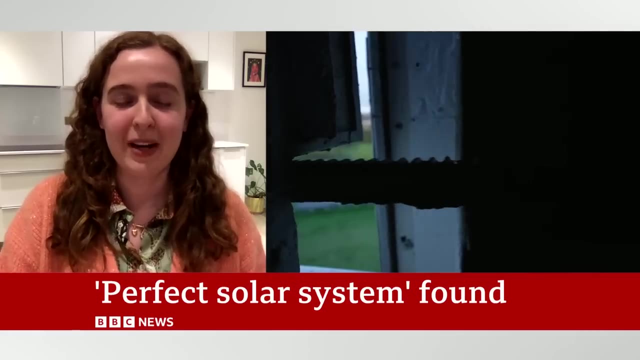 Yeah, Yeah. So this system, what we, what we did, was we used a NASA Space Telescope to observe the star And what we saw was that the star occasionally got slightly dimmer, and that tells us that there's probably a planet there. And what we found in this case was that we had signals of six different planets, and it took some. 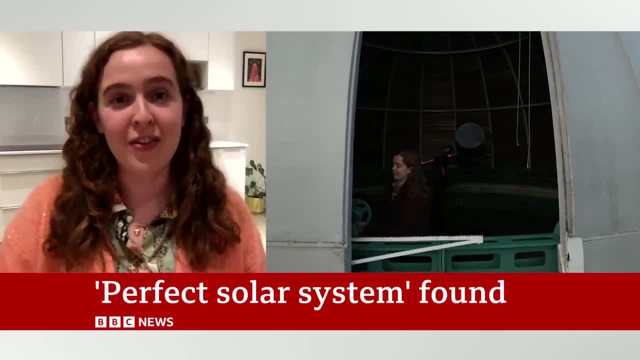 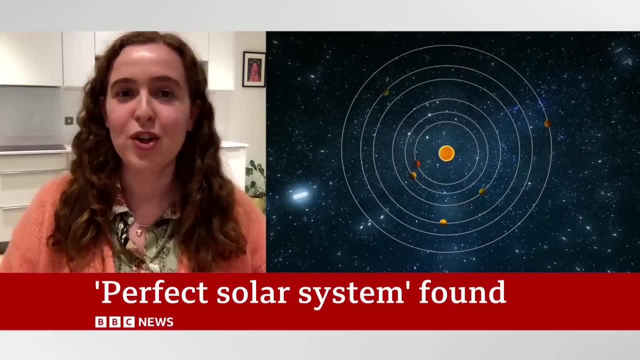 detective work. But after quite a lot of input we figured out that there were six planets and we figured out that they span sort of differently distances from the star. so we have some which are quite close to the star about a nine-day orbit, which is very hot, and we have some which are a bit further. 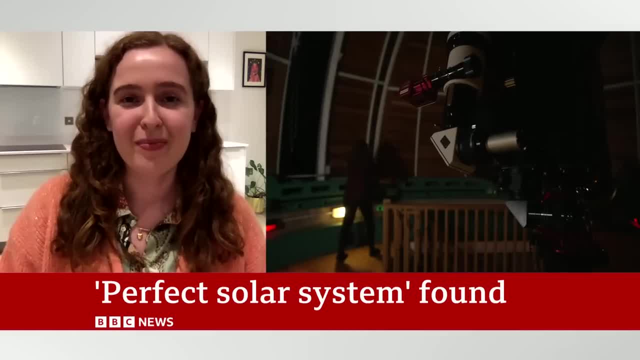 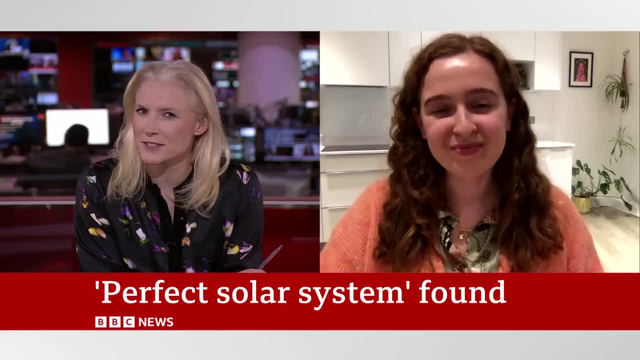 away on a 60-day orbit which are a bit cooler. but when you say a bit cooler, I think that the coolest is about 600 degrees, isn't it? and in terms of what that means for potential life, what, what is that? yeah, so exactly when we say cool, 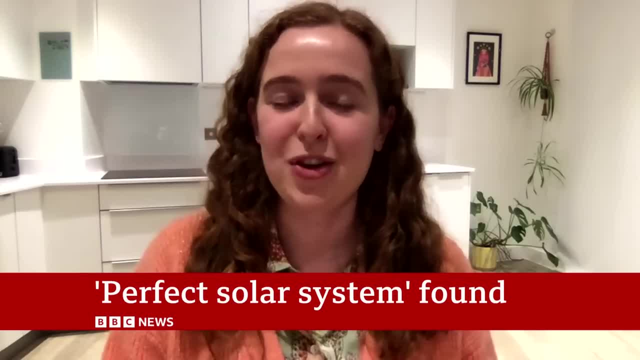 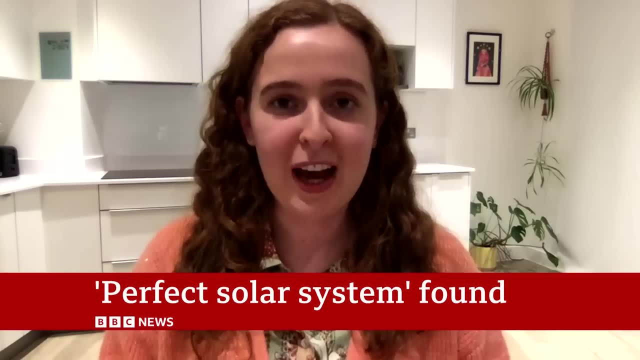 this isn't, you know, solar system temperatures. this is still much hotter than that, but it's interesting that we're being able to push out to these cooler planets that are going to be more amenable to life. and the interesting thing with this system is we have six planets so far, but there's nothing to 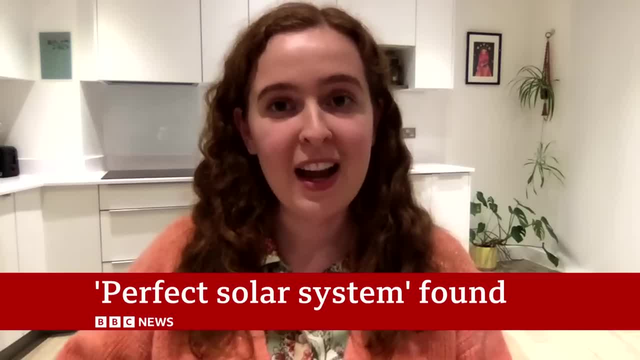 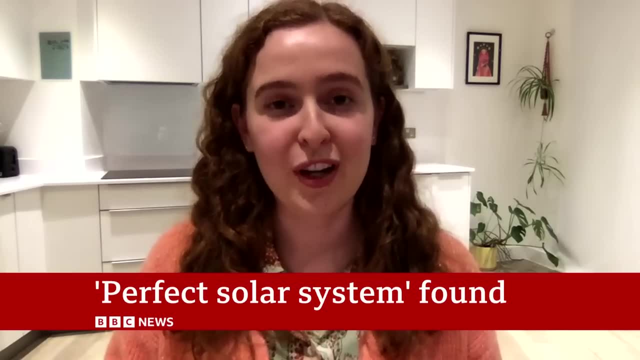 say that there might not be more planets further away from the star, and then these could be in the special region which we call the habitable zone, and that would be where liquid water could potentially exist on the surface of these planets. right, so you've done this, is your PhD already, but this is pretty. 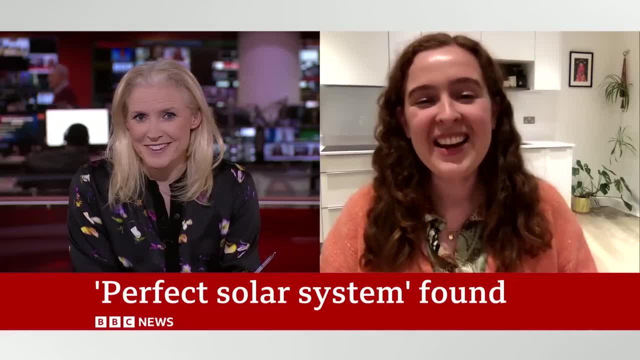 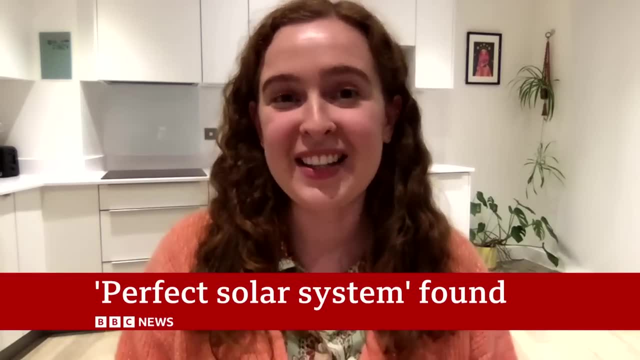 much going to take up the rest of your time forever, isn't it? so yeah, so this was led by one of my collaborators in Chicago and I've been contributing from one of the ESA telescope sides. but, exactly like, this is a really exciting system to continue working on in the future. I know. 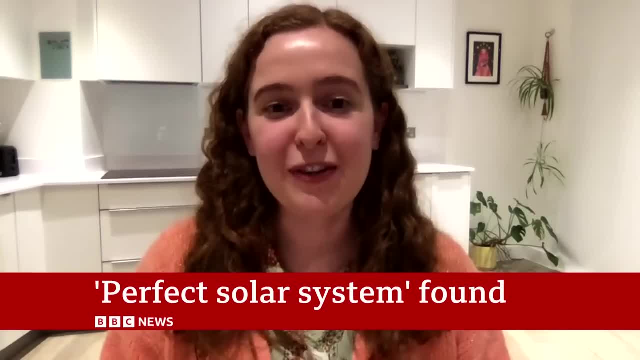 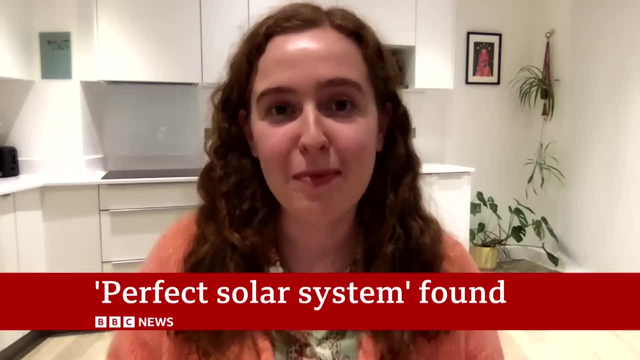 many of my collaborators are already doing additional studies, especially, for example, this is going to be perfect for the James Webb Space Telescope. so the James Webb Space Telescope is able to look into the atmospheres of the planet, which is incredible. like to think that we could figure out what is in the 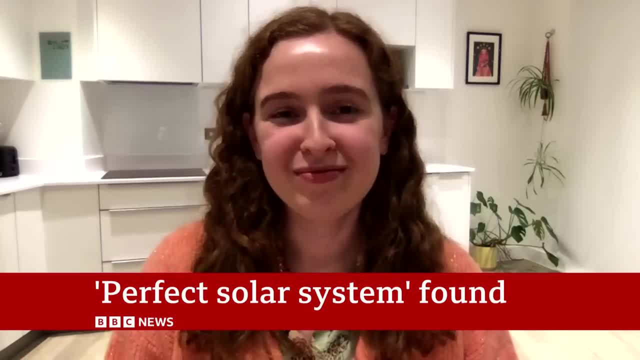 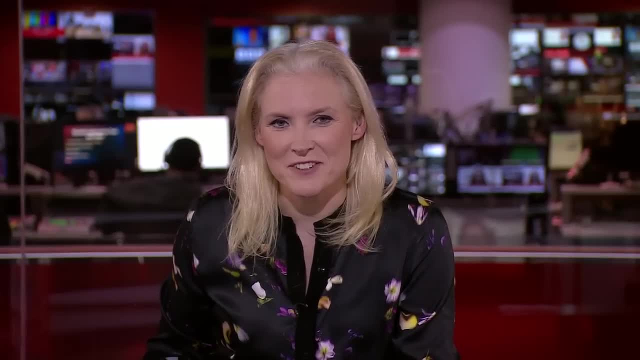 atmosphere of these planets hundreds of light years away. it is, it's extraordinary well. thank you so much for talking to us about it. it's lovely to hear from you. thank you, that's Amy Toussaint, PhD student at Cambridge University. thanks so much for your time. 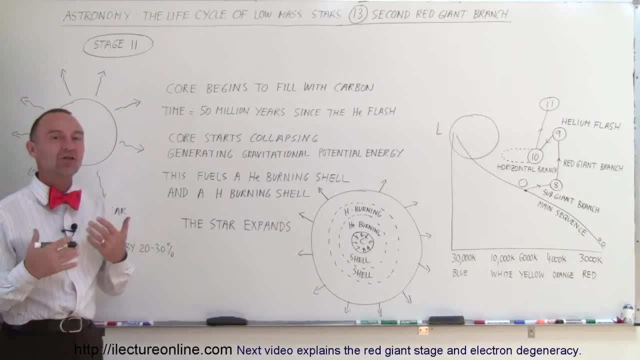 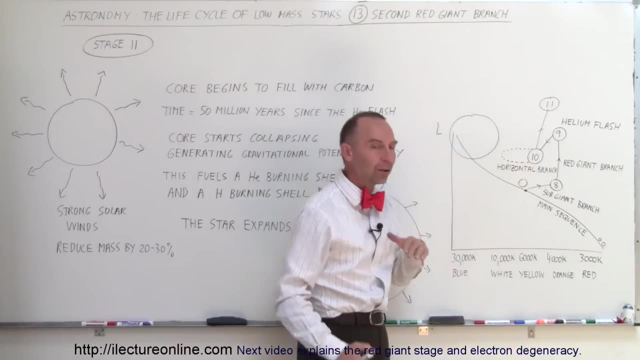 Welcome to ElectronLine, and now we're going to talk about the second red giant branch. What is taking place now? Well, the star is where we left it off on the last video, at the horizontal branch. This is kind of like the second main sequence stage of the star. The first main sequence stage is when the core was fusing hydrogen into helium. The second- quote main sequence stage would be the horizontal branch where the core is fusing helium into carbon. Now that process is much more ferocious at much higher temperatures- temperatures above 100 million degrees Kelvin- And so this process happens to be so quick. that that stage only lasts about 50 million years. For the sun, the main sequence stage lasts 10 billion years, but the horizontal branch stage, where it's a red giant burning helium into carbon, it only lasts about 50 million years, And the bigger stars it's. even less. For the very large stars that process may only take about 10 million years, And for smaller stars in the sun it could take more than 50 million years. But eventually the whole core begins to fill with carbon, And once that happens the fusion process from helium to carbon tends to slow down. 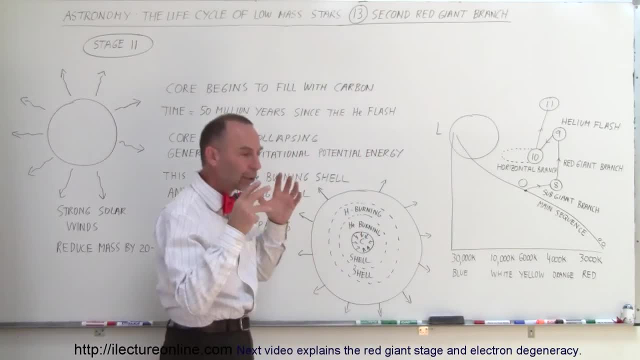 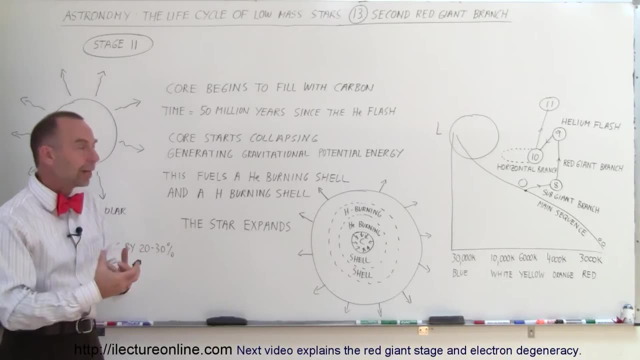 from burning hydrogen to helium. when that process ended and the core began to collapse. this is a very similar process: Gravity again takes over, begins to collapse the core, That heat generated due to what we call the gravitational potential energy being converted to heat fuels the 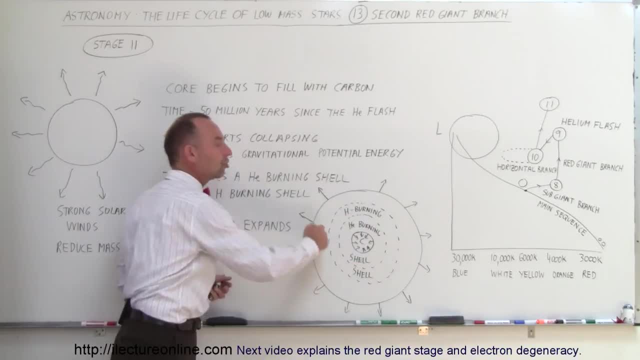 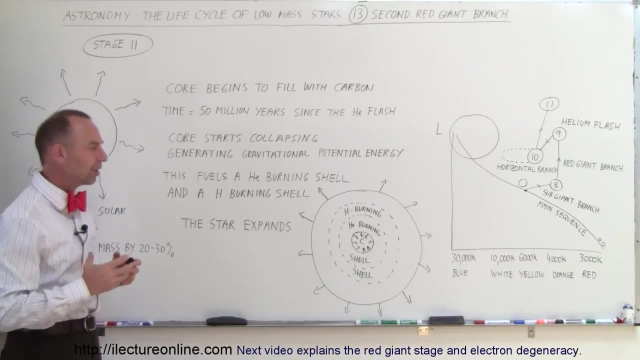 helium burning shell around the core and the hydrogen burning shell around the core. So that is still ferociously taking place because the energy being generated from the core collapsing, all that extra heat being generated, and because of that additional heat being generated, the star begins to expand again.